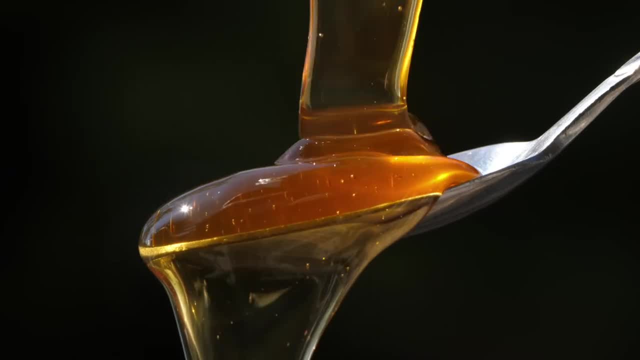 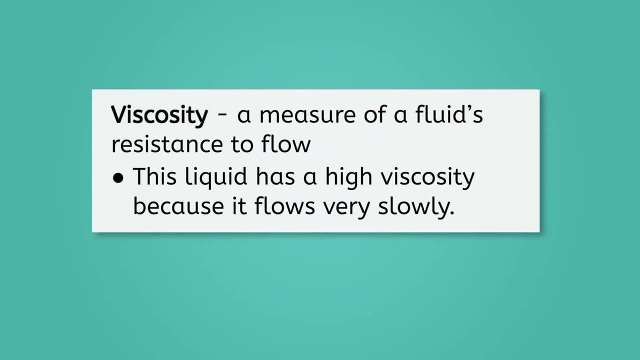 it is thick and moves slowly, meaning it has a high viscosity. Viscosity is a measure of a fluid's resistance to flow. If you think about those two properties- golden color and a thick, slow flow- can you narrow down the identity of the substance to a few options? 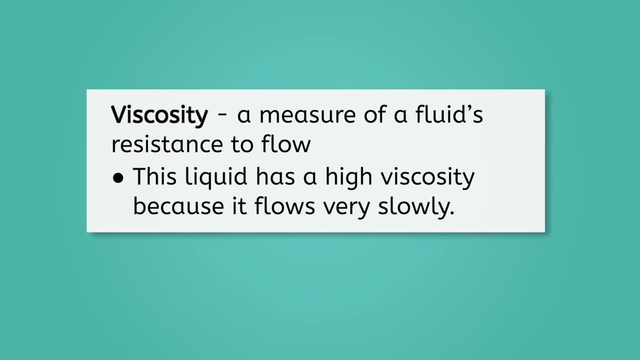 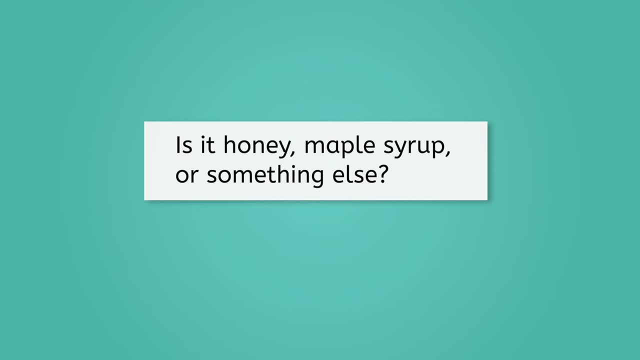 Given those two properties, it could be honey, maple syrup, and maybe there are a few other substances. it could be too. If we really wanted to further narrow it down, we could test its density, boiling point, etc. Eventually, we would be able to confidently say that the liquid is honey. 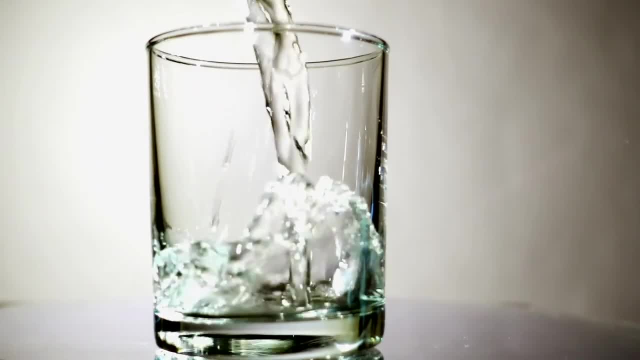 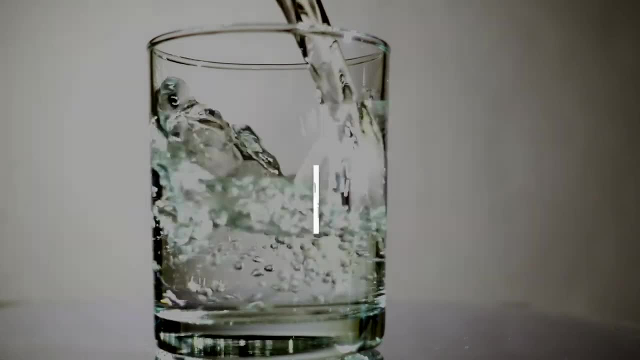 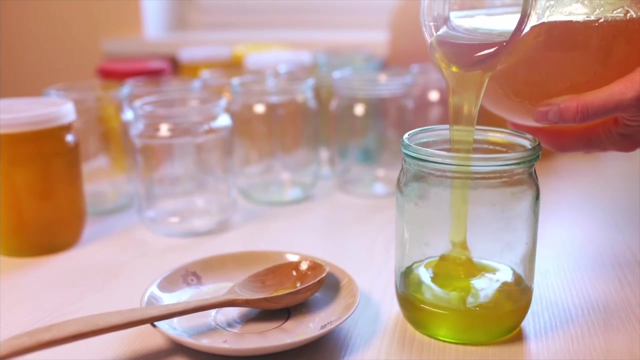 When describing a substance, there are a multitude of properties that can be used and the liquid is honey, And the combination of those properties is unique to every substance. For example, water would have very different properties from this honey, like lower viscosity and a colorless appearance. Some properties can be seen. 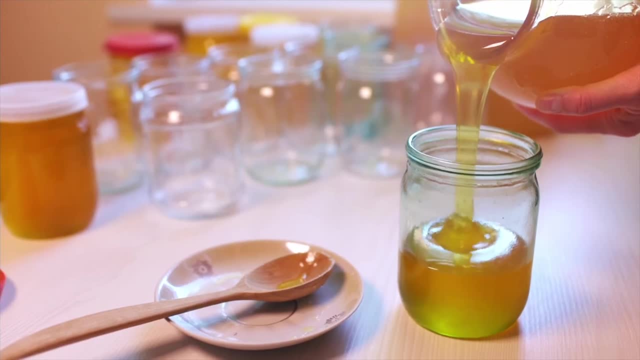 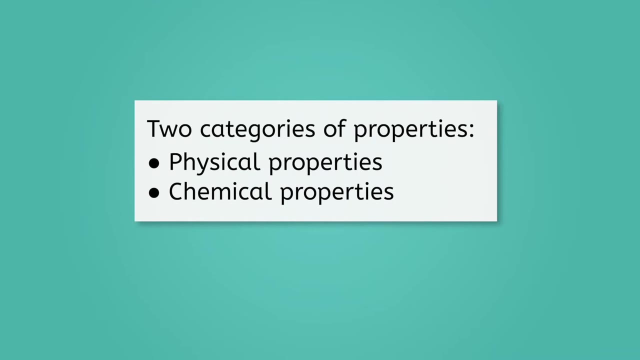 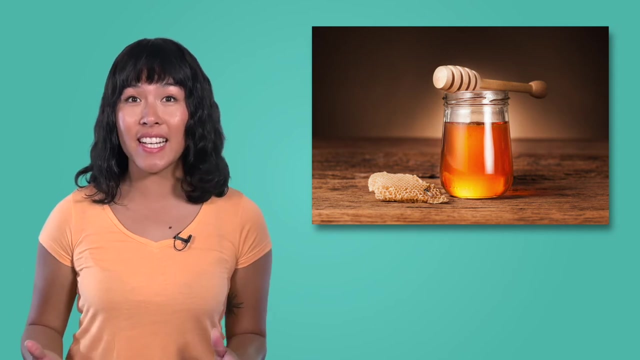 while others must be tested or observed in experiments. All properties fall into one of two categories: physical properties and chemical properties. Think back to the honey. earlier in this lesson we were able to easily describe its color and viscosity. Color and viscosity are examples of physical properties. 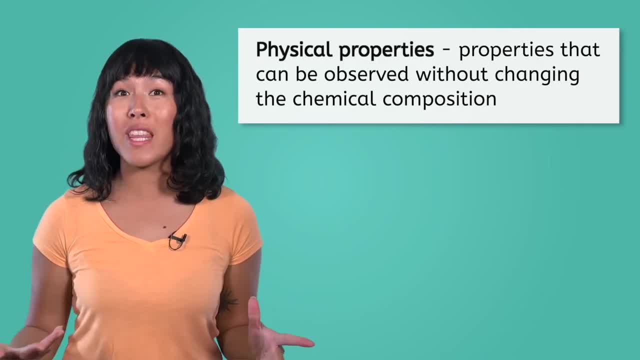 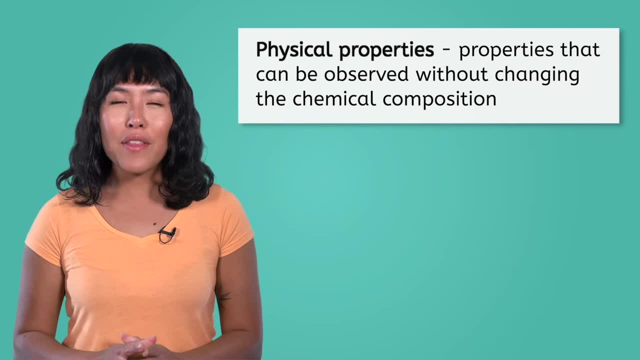 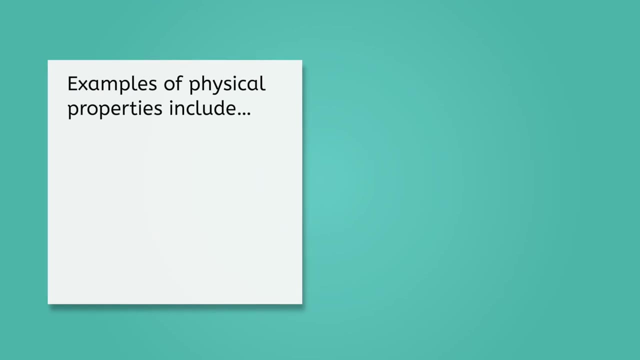 Physical properties are properties that can be observed without changing the chemical composition, meaning you don't change what the substance is, but rather make observations based on what you see. Can you think of some more examples of physical properties? Some examples include color, shape and mass. 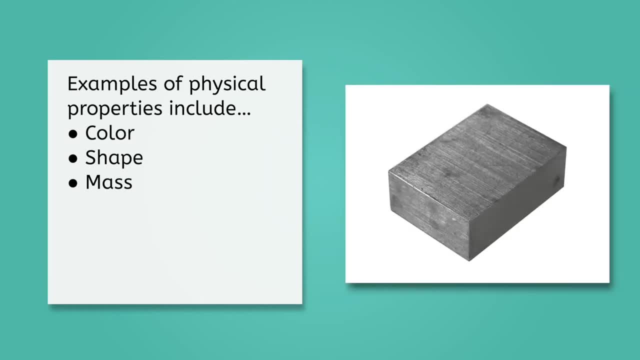 What about density? Can you find the density of this metal without changing it? Yes, you can, by calculating the volume and measuring the mass. What about boiling point and freezing point? Using a thermometer, you can measure the boiling point and freezing point of a liquid. 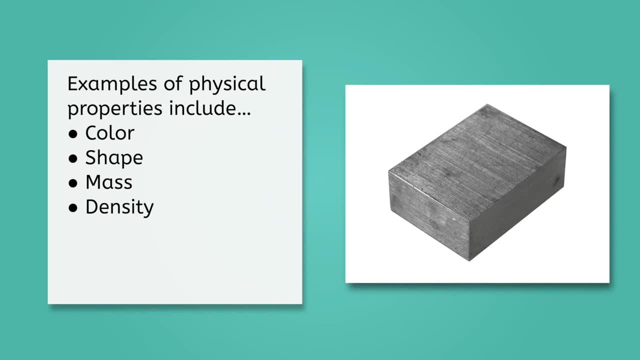 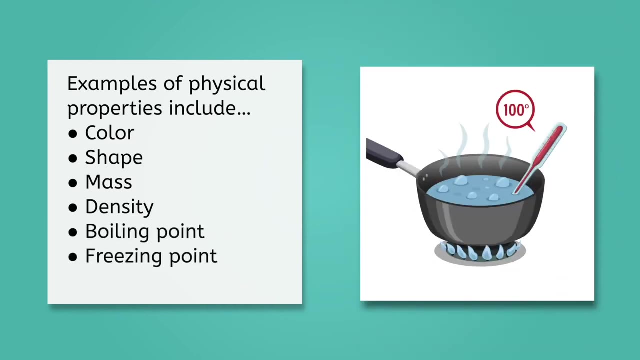 and, as we learned in a previous lesson, there is no change in the substance during phase changes. The particles are just moving slower or faster, causing the state of matter to change. This means that boiling point and freezing point are also physical properties. 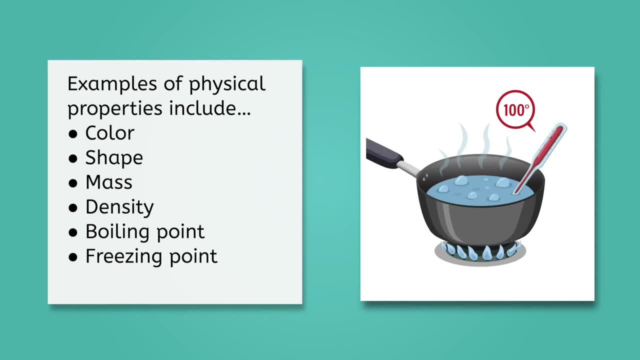 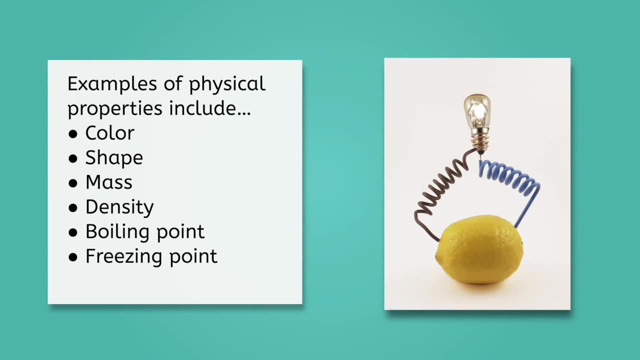 Another example of a physical property is the ability to conduct electricity. Have you ever tried the good ol' lemon or potato as a battery electricity experiment? In these situations, the lemon or potato are not changing while the electricity flows through them. This means conductivity is a physical property. 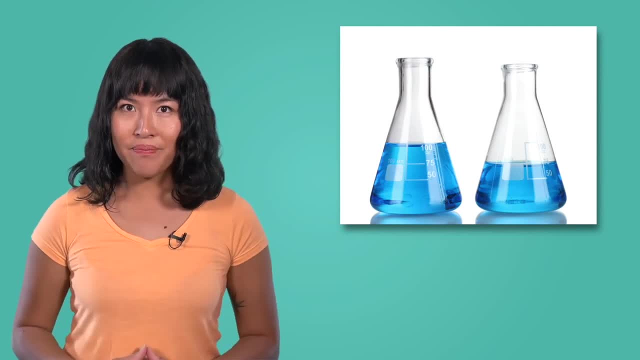 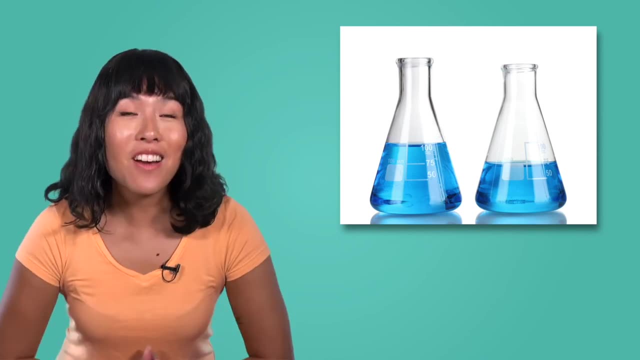 These two flasks contain the same exact liquid. Looking at them, we can determine two physical properties: color- blue- and volume. The flask on the left has a volume of 100 milliliters and the one on the right has a volume of 75 milliliters. 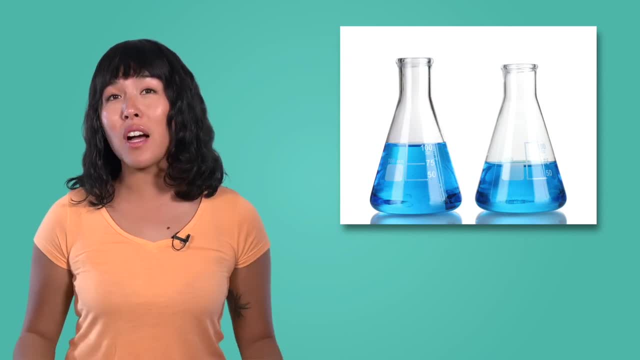 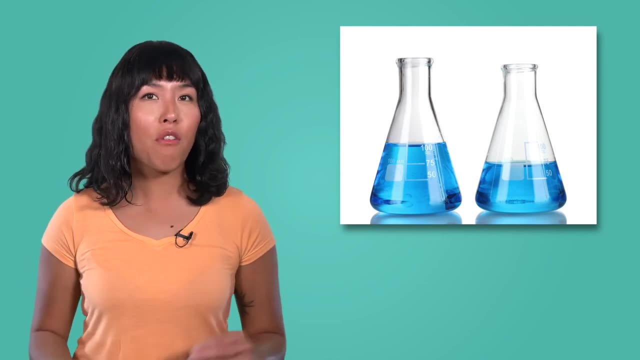 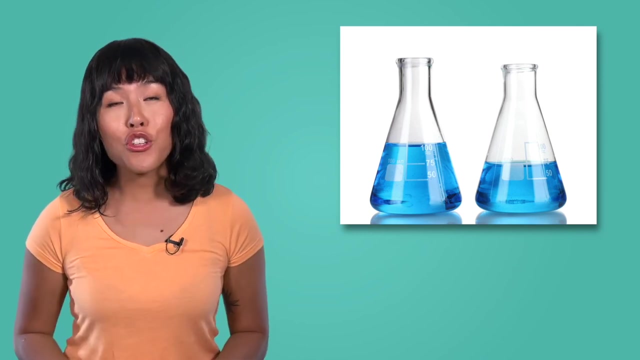 75 milliliters. Even though both color and volume are physical properties, when the amount of the substance changed, the color stayed the same, while the volume did not. Color is a specific type of physical property called an intensive property, while volume is an extensive property- All physical. 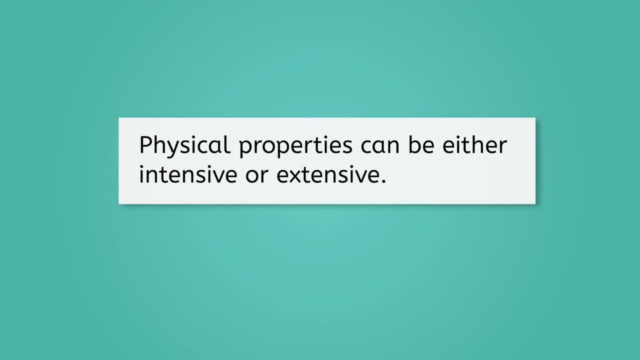 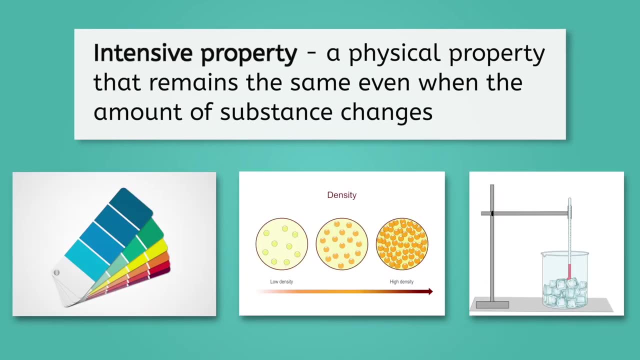 properties are either intensive or extensive properties. Intensive properties are properties such as color density and freezing point. These are all properties that remain the same no matter how much of the substance is present. On the other hand, mass and volume are examples of extensive 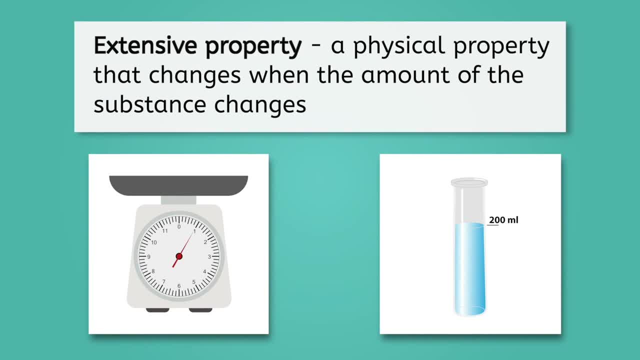 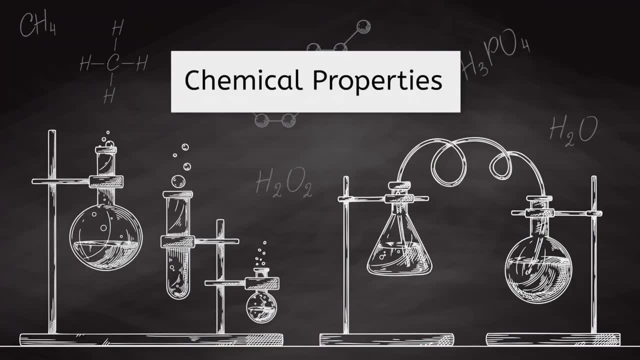 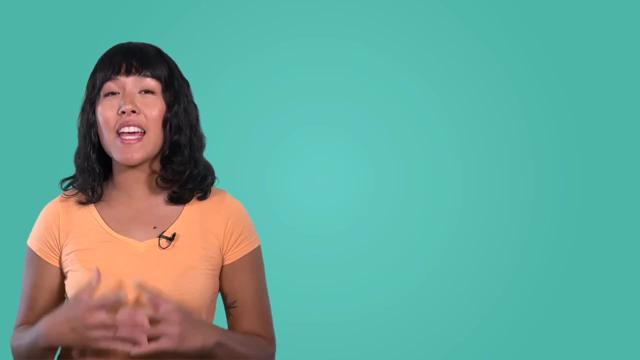 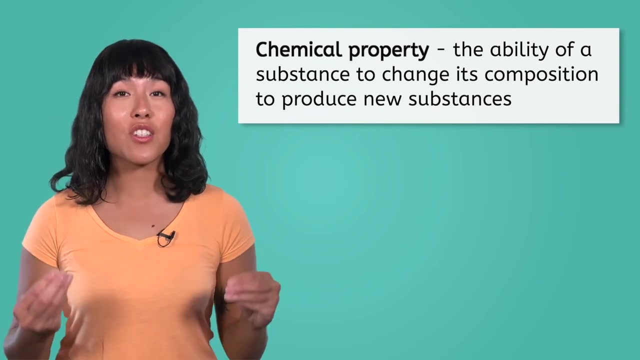 properties. These are properties that depend on the amount of the substance and will change accordingly. A substance's chemical property is a chemical property that is not a substance. Chemical properties are a little harder to notice than its physical properties. A chemical property is the ability of a substance to change its composition to produce new substances, meaning 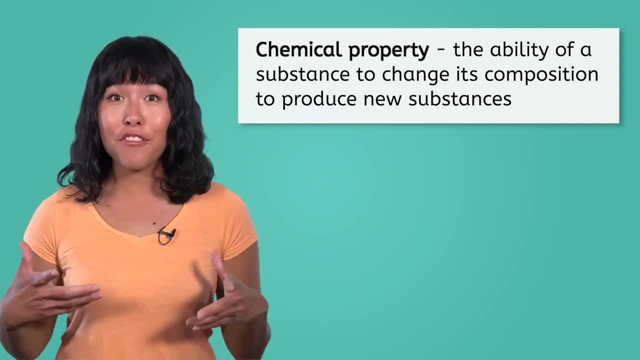 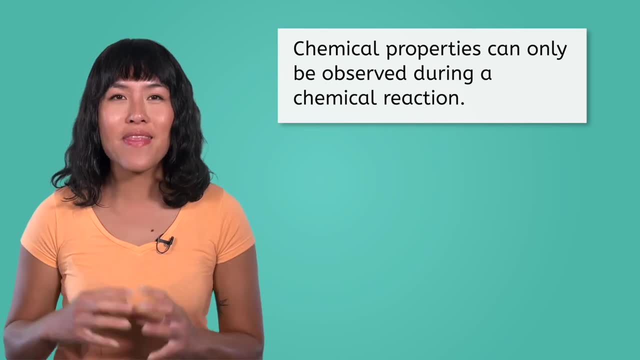 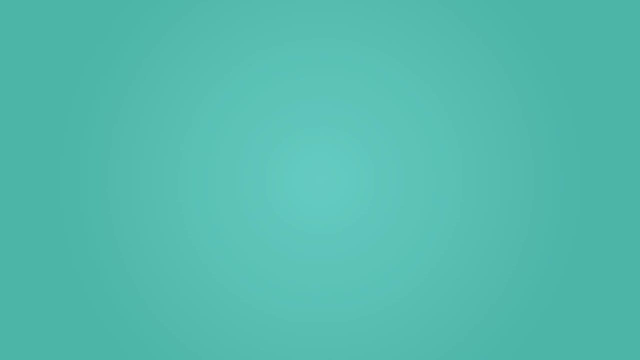 that at the atomic level you end up with a different substance than you started with. That means chemical properties can only be observed when the chemical composition of the substance changes. Chemical properties include a substance's reactivity with other chemicals such as water and oxygen. its